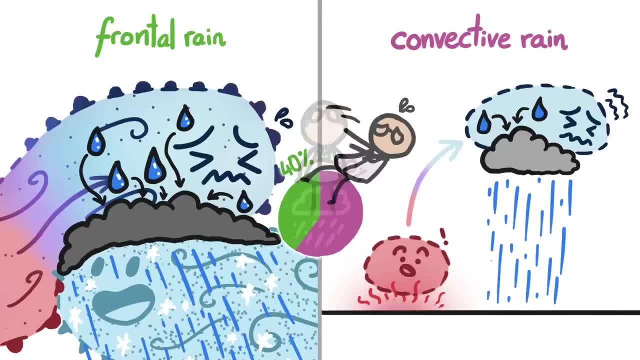 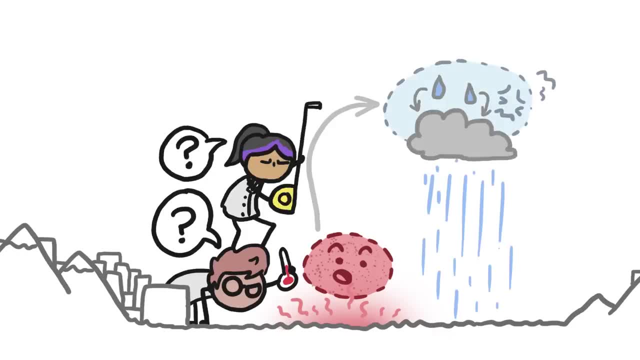 rather than the temperature difference between two large masses of air. it's much more complicated. It's hard to know how warm various parts of the ground will be at a particular time, whether that heat will be enough to lift a particular mass of air to a particular height. 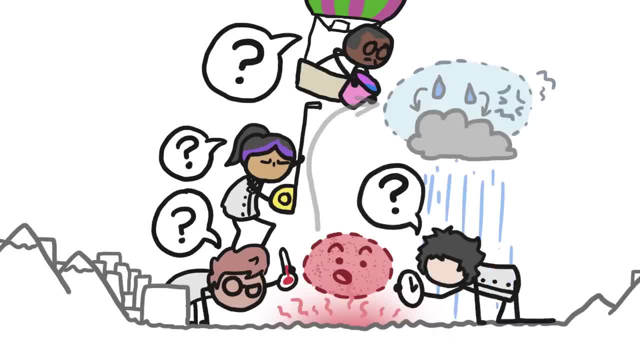 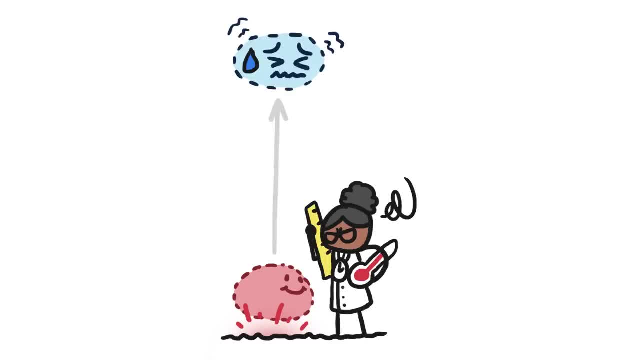 how much water vapor that particular mass of air holds and how long that particular mass of air will stay over that particular patch of warm ground. As a result of all these variables, rain from convection can look like a light sun shower or a severe thunderstorm. 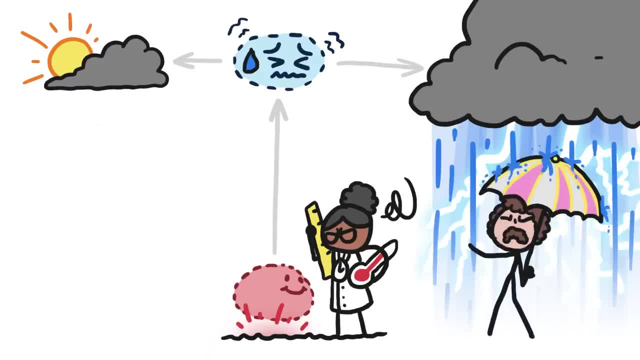 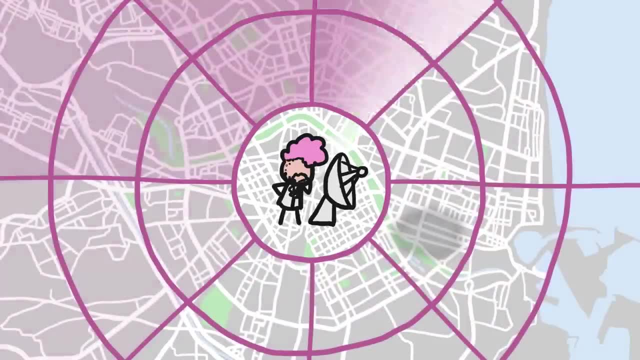 and it can be over in minutes or last for hours. What's more, the masses of air involved in convective rain are often way smaller than the resolution of most meteorological monitoring systems. So not only are the many storms hard for radars to detect, 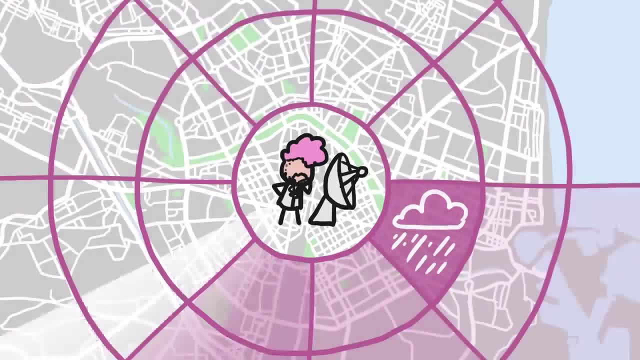 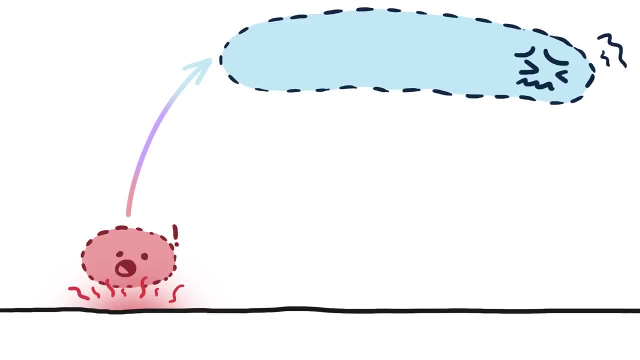 but even if the storms do get detected, meteorologists have no idea if it's raining in the whole area or only parts of it. And here's the extra frustrating thing about this hard to predict type of rain, because it gets kicked off when the ground gets heated. 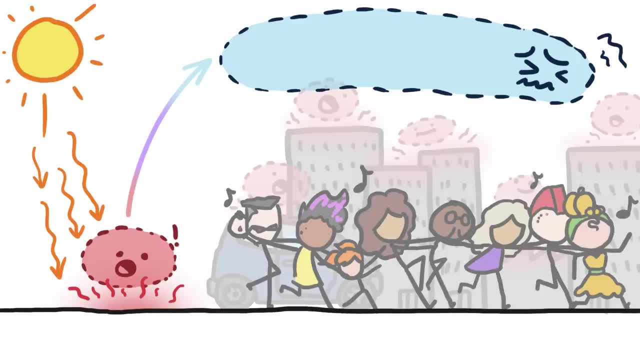 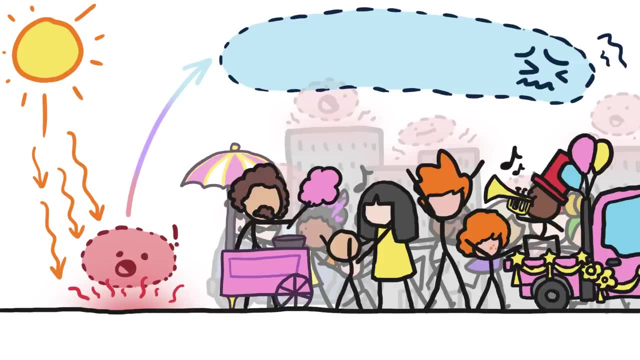 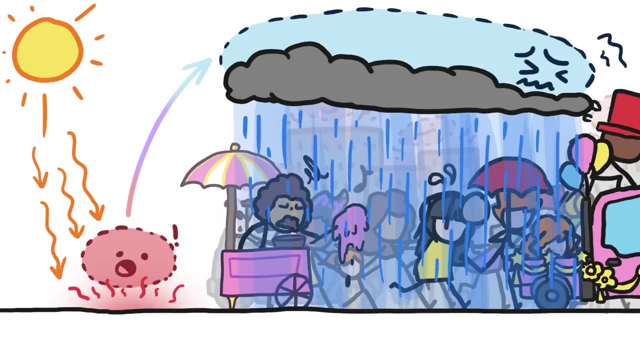 It's way more likely to happen in the summer and in places with lots of heat absorbing materials, like cities. So when this type of rain does fall, it's often at a time and place where lots of people are gathering together outside. In other words, it's not all that uncommon for it to literally rain on your parade. 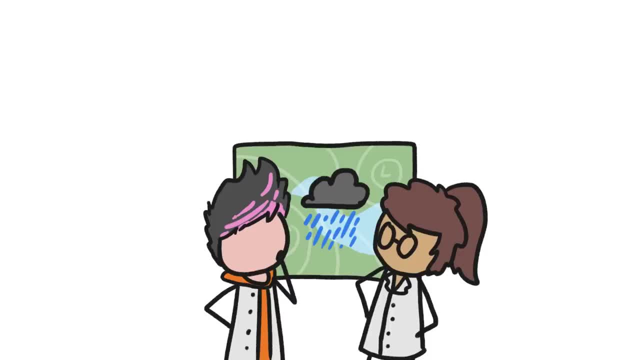 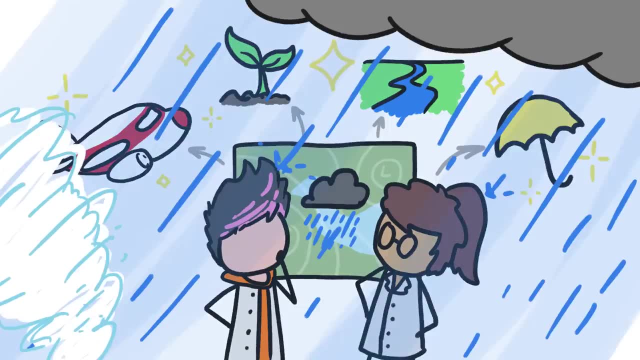 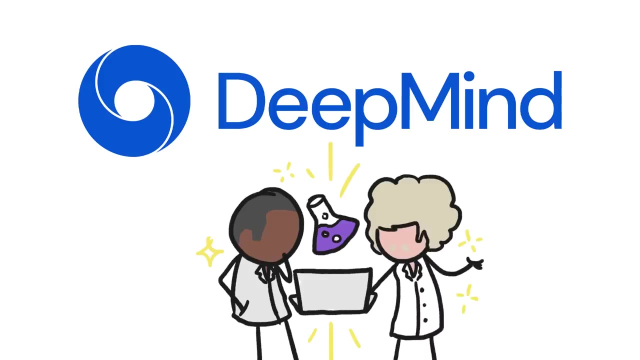 More accurately predicting rainfall will help us with all sorts of stuff: Air travel, farming, water management, emergency planning and, more especially, as the weather gets more extreme. That's where this video's sponsor, DeepMind, comes in, an AI research lab working on some of the hardest problems in science. 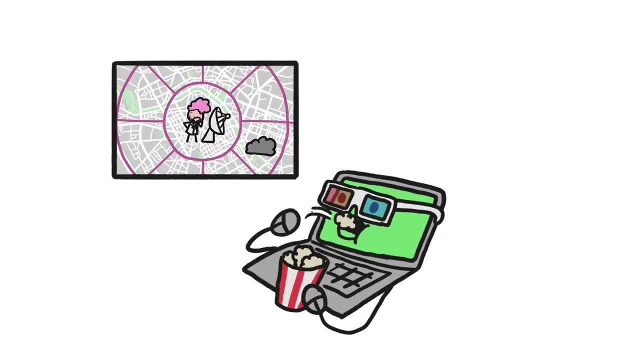 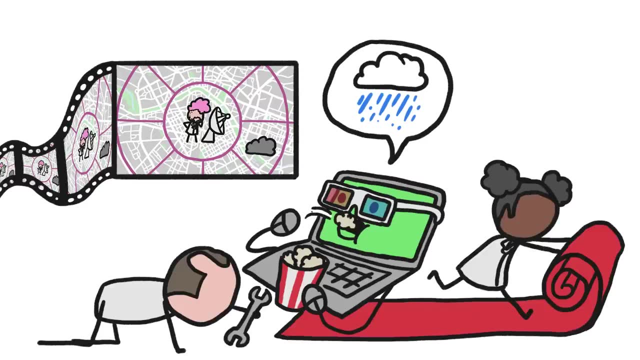 DeepMind's weather forecasting AI treats radar data like a movie, predicting the next few frames in the scene based on what's come before. Even though researchers are still working to get this technology ready for prime time, they've seen huge increases in the accuracy of short-term weather forecasts. 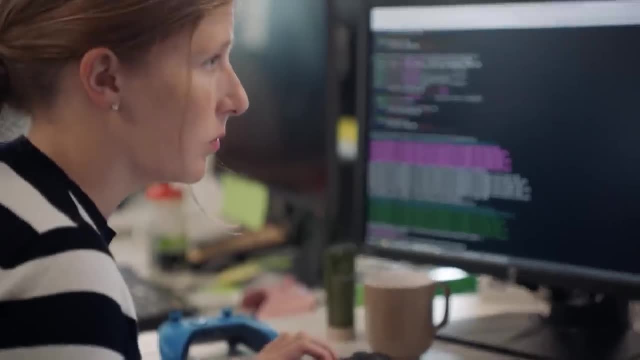 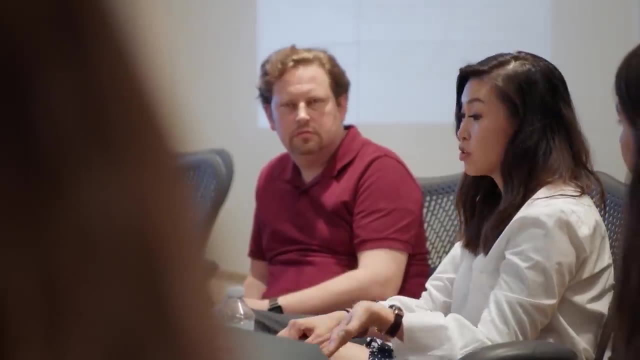 If AI is going to benefit everyone, the researchers and engineers working on it must have diverse perspectives. So DeepMind has created a scholarships program to provide financial support, mentorship and more to students from underrepresented groups seeking to study AI or a related field.